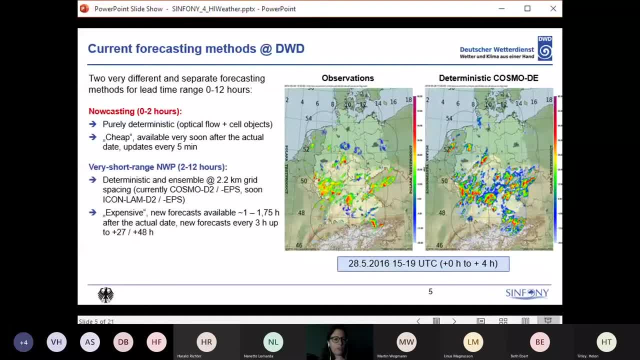 Updates every five minutes. For very short-range NWP we use deterministic and ensemble high-resolution model, Currently still our COSMO D2 and EPS and soon we will have an ICON LAM version. here Again, you see on the right-hand side the observation and a deterministic COSMO forecast. 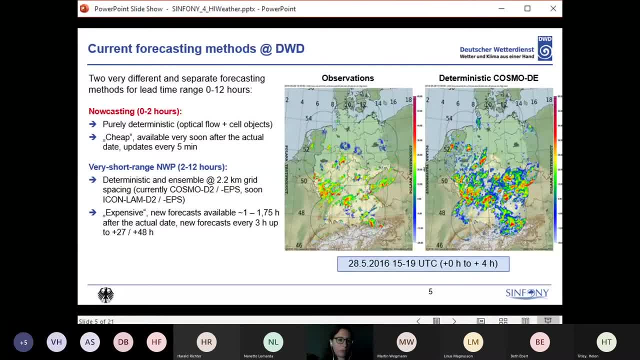 These methods, of course, are rather expensive. New forecasts are available only 1 to 1.75 hours after the actual date. New forecasts are set up every three hours and run to plus 27 or plus 48 hours. Up to now, these methods have been developed quite separately, and there also exists no common products. 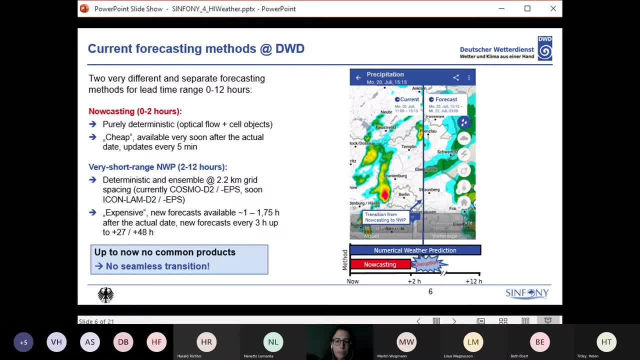 So this means we do not have- We do not have a seamless transition, and this also exemplifies in our WarnWetter app, which is shown here on the right. So this is basically what the users outside get on precipitation fields and on the left part you see what stems from now casting. 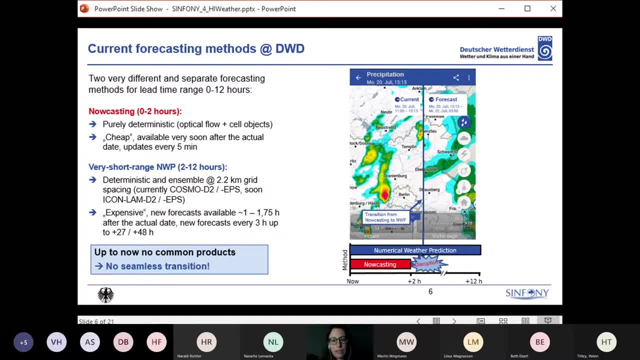 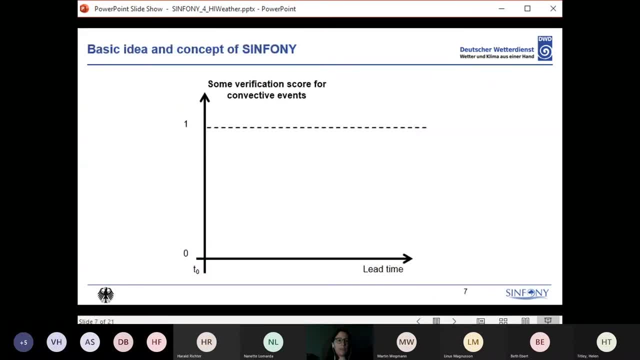 On the right. you see what stems from the NWP and you clearly see that there is a real cut between the two And this cut We want to eliminate as good as possible with our symphony system. so the basic idea can be explained on this score plot. so you assume some verification score for convective events. 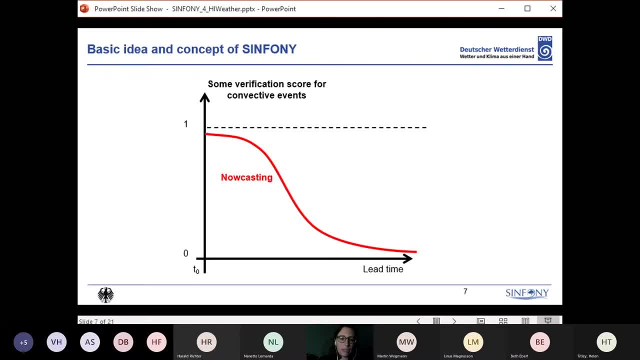 We have the now casting, which is really good, performing at short lead times, but drops down at later lead times. You have NWP, which starts earlier than the actual date, which is initialized earlier than the actual date, Starts with a lower score but at the end outperforms now casting at longer lead times. 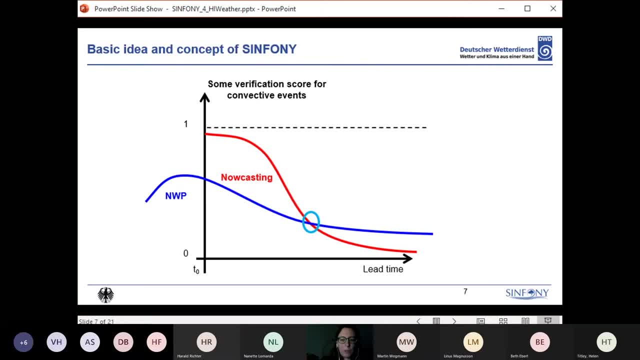 And at one point you have the intersection where both show the same score. On the one hand, with Symfony we now aim to improve our now casting methods themselves. We also want to improve and expand our NWP, So with overall we get a better skill of both of them. 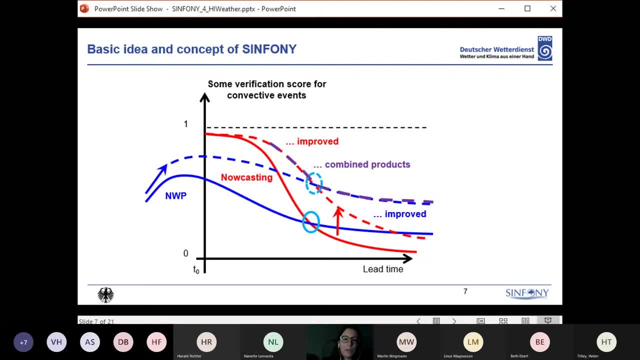 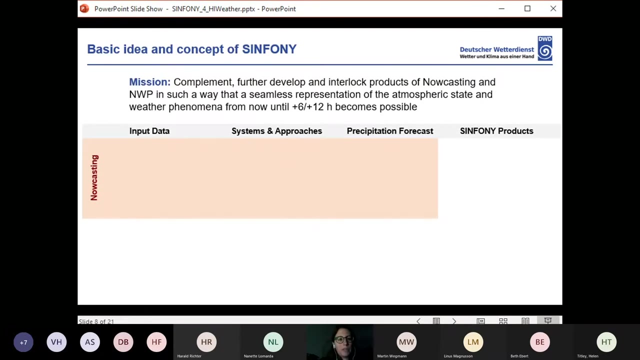 And Then we also develop some combined products that seamlessly bring together the best information from both worlds into a mostly seamless product. At the moment, the focus is put here on precipitation forecasts, And so the mission is to complement, further, develop and interlock products of now casting and NWP in such a way that a seamless representation of the atmospheric state and weather phenomena from now until 6 to 12 o'clock 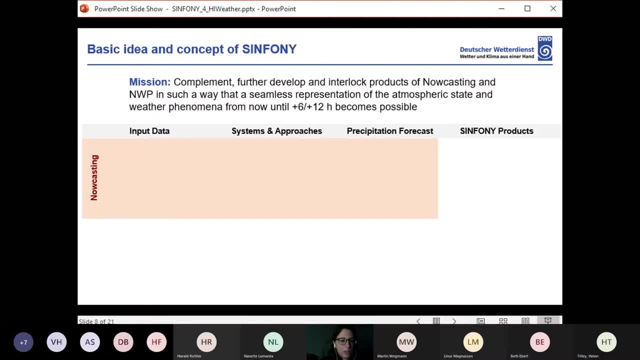 becomes possible For the now casting this means. So in black you see the current data that is used for now casting and in red what's new, or in addition with Symfony. So we want to switch from two dimensional to volume radar data. 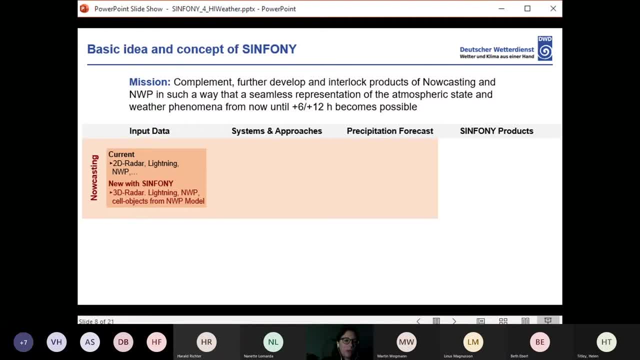 We also include lightning And we also include cell objects from the NWP model. So with cells we mean convective cells that have been identified by an algorithm in the NWP forecast. So this cell algorithm detection is something that we usually use for now casting. 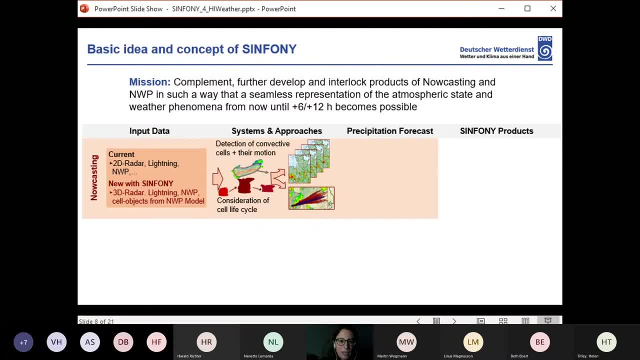 I will come to it in a minute- and we will now also employ it on model data. Then the system and approaches are, on the one hand, an optimized optical flow and switching from a deterministic to an ensemble ansatz. here, And also for the cell objects, we consider the typical life cycle of convective cells. 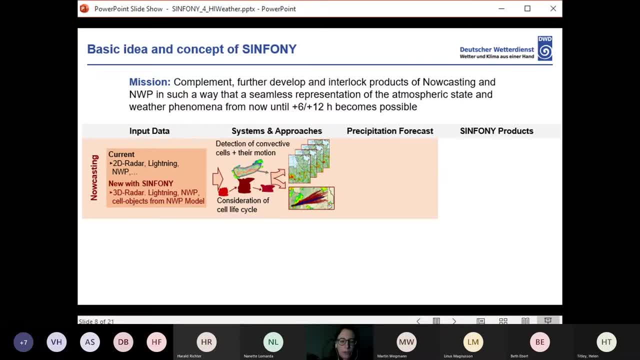 and try to get an estimate about the future intensification or weakening. This means our future precipitation forecast for the now casting part will be a now casting ensemble for gridded field precipitation and also for cell objects from zero to six hours For the 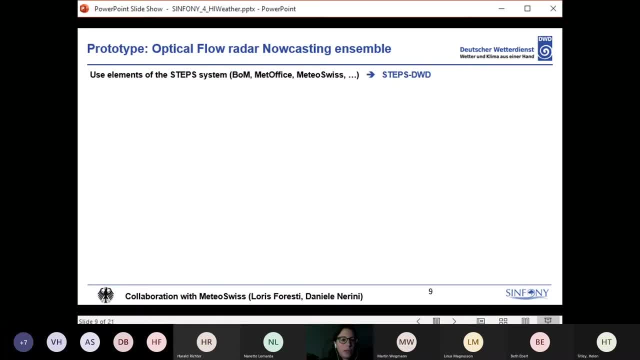 optical flow radar, now casting ensemble. we use elements of the STEP system that has been used at many other weather services already and some of you might be familiar with it. We call it STEP-DWD because we have made some refinement concerning localizations. 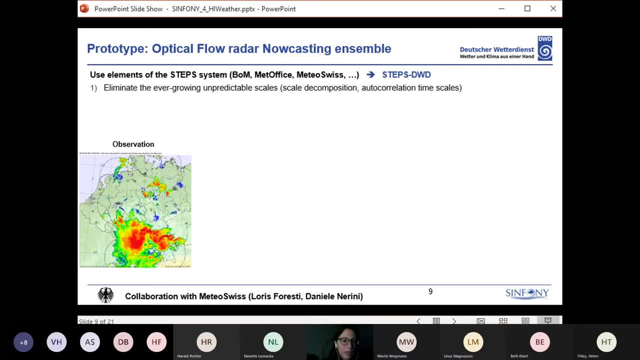 So the basic idea of this approach is: you have the observation from the radar data. There you eliminate the ever-growing unpredictability and you see the same level of predictability that we were talking about, And then you can. you can see that the model and the objective data is usually very similar. and the objective data is supposed to be very similar as well. And then you get a graph and then a graph of a population, and then you get a graph of a population and then a graph of a population and then a graph of a population. And then you get a graph of a population, which is the time period where "'I'm not sure what the data is, but what is your prediction of the results of that and how many of the data? we call it and what is in that? 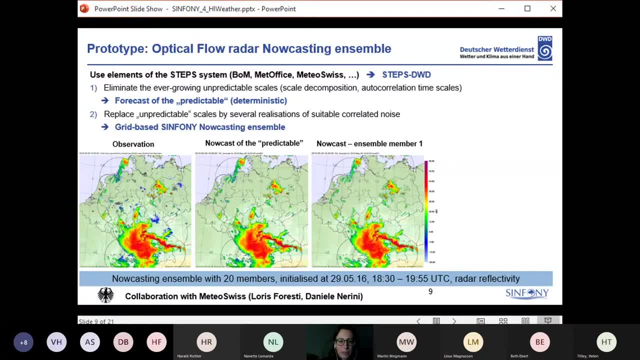 when you have a input of the data is removed, and what is the data that you are considering? In the middle is now shown one ensemble member as an example, And we run this with 20, sometimes also with 30 or 40 members. 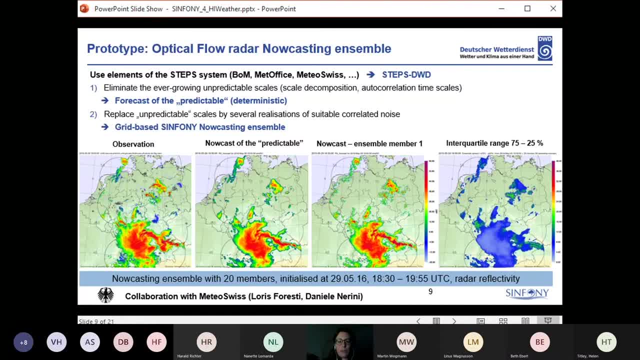 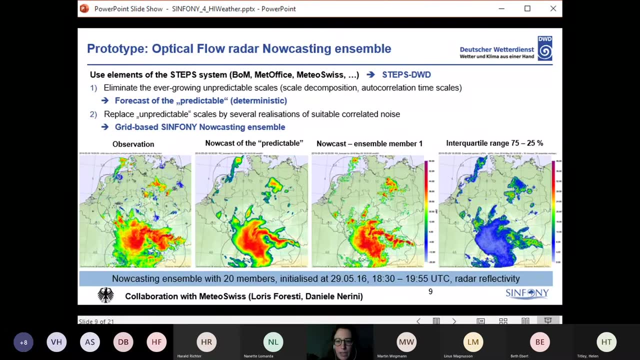 We will see how many we can afford in the end. And this ensemble then also allows you to derive information about ensemble spread, which on the right hand is shown now, and in particular the regions and the boundary regions of these convective events. These are prone to larger ensemble spread in that case. 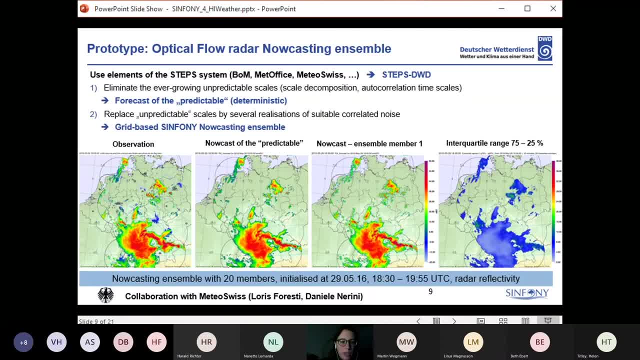 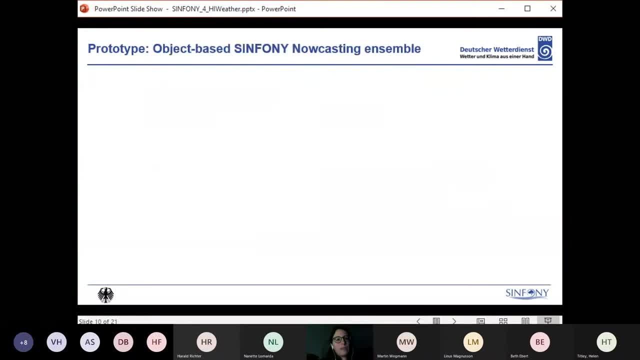 And this is also a collaboration we are doing together with colleagues from Meteo Swiss, and also want to thank them for their support here. The other one is the object-based symphony, now casting ensemble, I talked about already. This is based on our Conrad 3D. 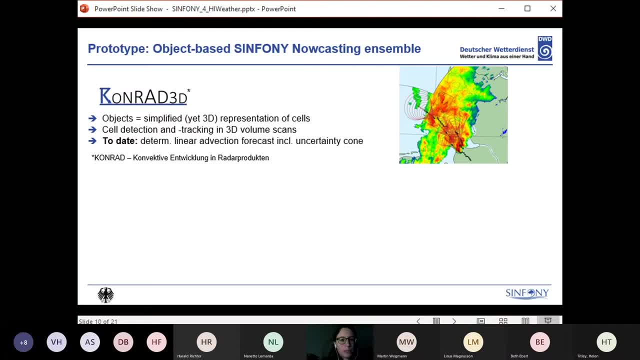 So objects is kind of a simplified but still a three-dimensional representation of a convective cell. Then we use a cell detection and tracking algorithm applied to our 3D volume scans of the radar. Up to date this is just a deterministic linear advection of the cells. 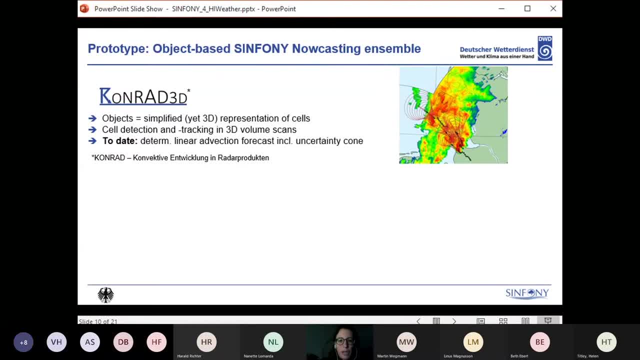 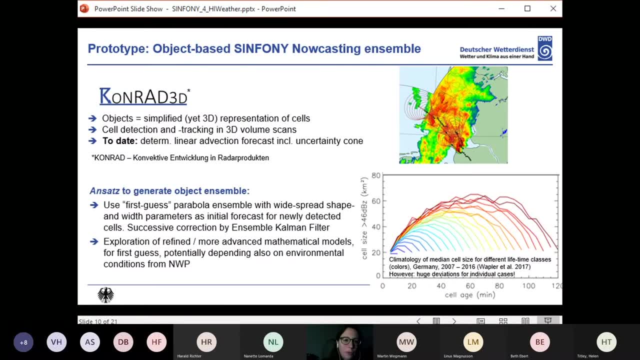 but also with some uncertainty, cone information. This is shown on the right And as part of symphony, now using first-guess parabolas, we have a parabola ensemble which kind of represents the climatological means median cell size for convective cells over Germany. 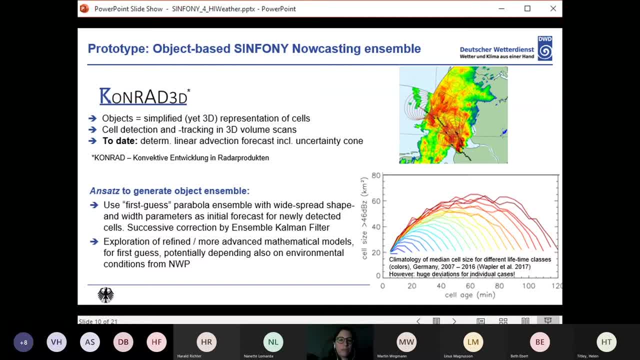 So there has been a study on which kind of line or curve represents best the life cycle of convective cells over Germany, And we found this parabola to be a pretty good first guess in some cases, And this is then also successively. 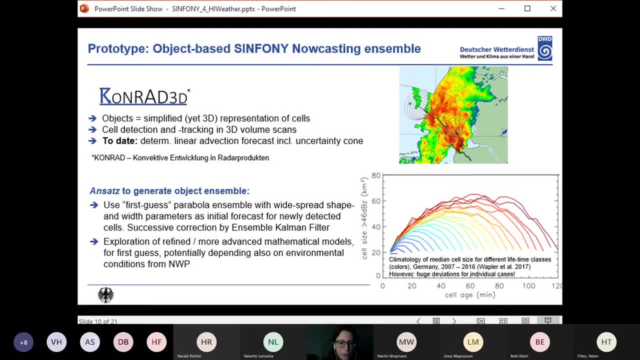 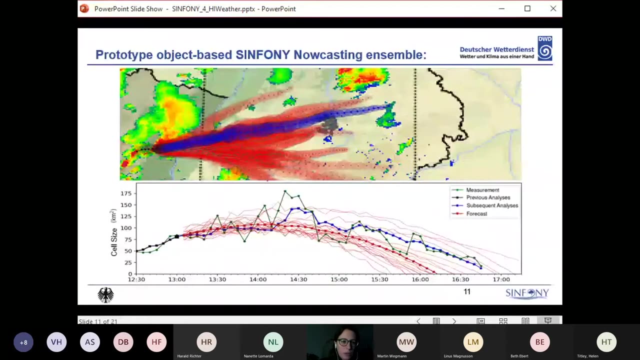 corrected by an ensemble Kalman filter. In the future, we also want to explore refined or more advanced mathematical models for the first guess, potentially also connected to environmental conditions from NWP. So here you see an example of this object-based symphony, now casting ensemble. 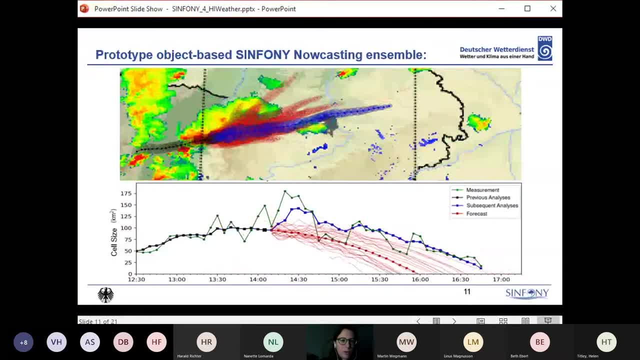 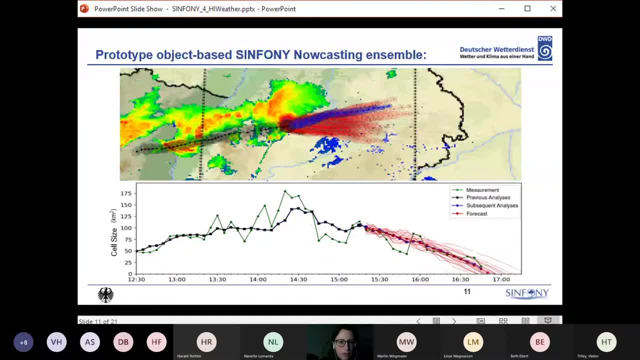 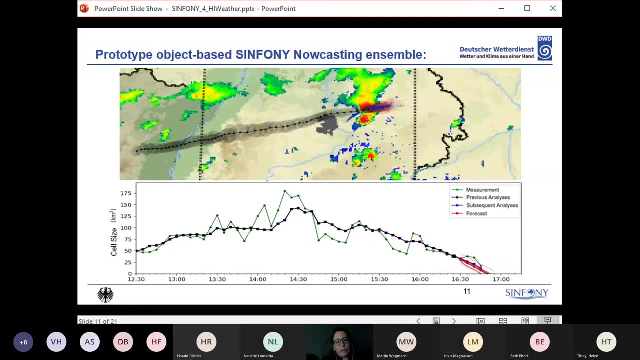 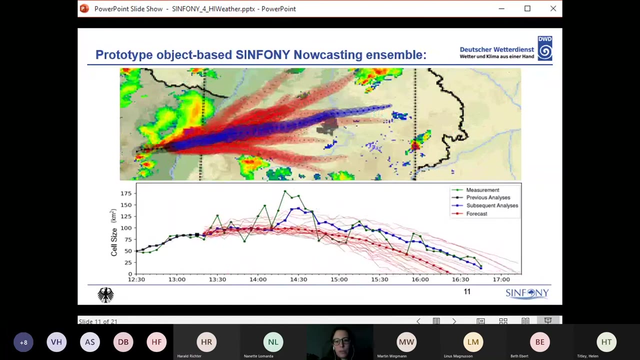 On the bottom you see the cell size and on top you see the ensemble. So this is kind of how this ensemble Kalman filter corrects for the cell size, And the red lines basically show where the different ensemble members propagate their cells And you can also then combine this information to make a probability to see what's the most probable. 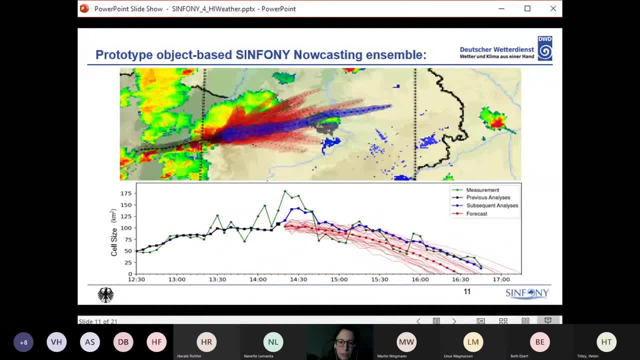 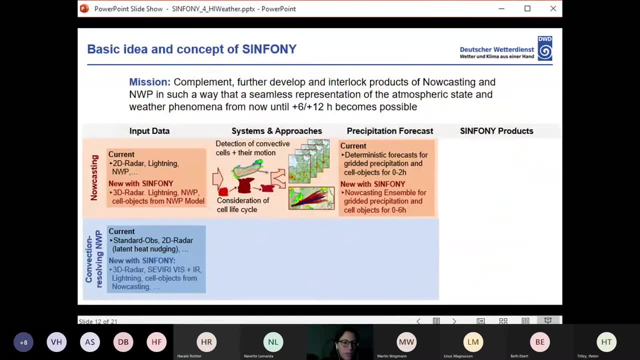 the most likely track the cell will take up in the future. So for the convection resolving NWP we will add information from Siviri satellite data. We also work on assimilating lightning And this makes the connection between now casting and WP. 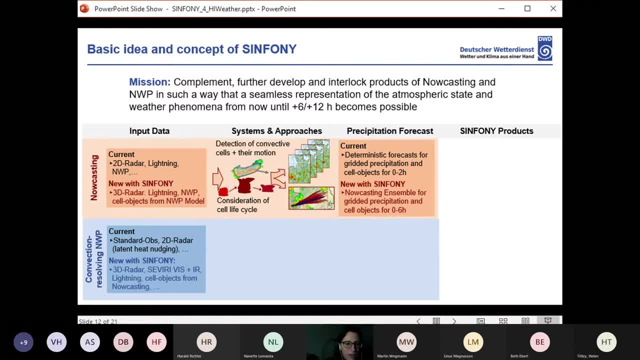 We also work on assimilating the cell objects we identified in the now casting. This will then put into our icon model, And we also work On setting up a so-called rapid update cycle version of icon. So it's an icon APS that will run every hour for 0 to 12 hours. 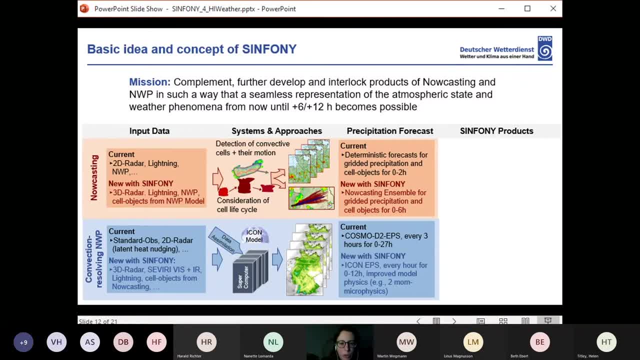 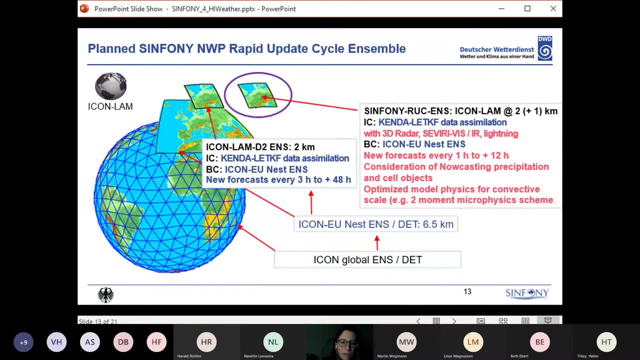 Also with improved model physics. For example, we are switching to the two-moment microphysics scheme here because it's a better representation there of the convective cells, as we found. So just briefly go through our model chains. So we have the global EU. 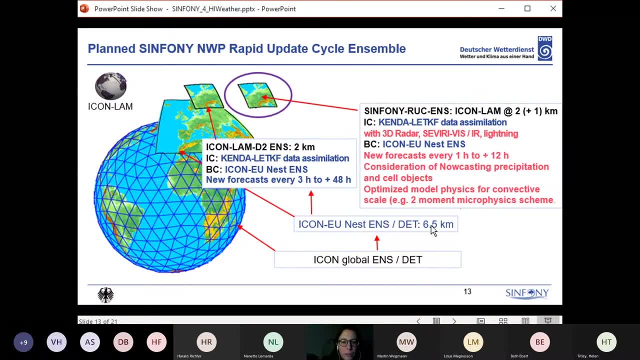 Then we have a global icon, Then we have the icon EU with 6.5.. Then we have the icon LAMD2 ensemble with 2 kilometers. So all of this will remain And in addition, we will have this Symphony Rook ensemble. 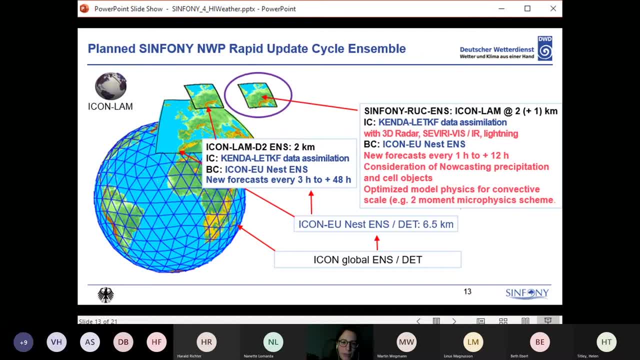 with basically what I said already: improved data from now casting Also satellite data, 3D radar data and so on, And this run will then also be available about 45 minutes after the actual data, not 1 to 1.75 minutes after initialization. 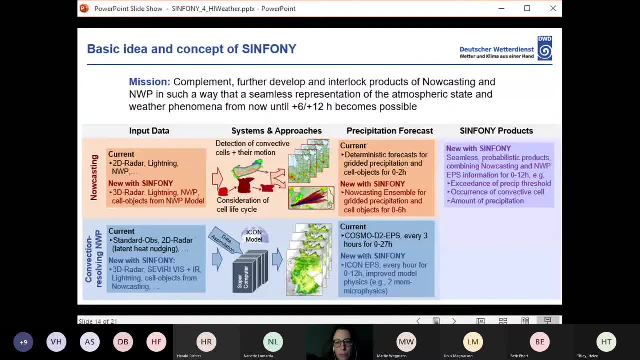 Concerning the Symphony products. So we work on seamless probabilistic products that combine the now casting and NWP EPS information from 0 to 12 hours, And these products will then, for example, allow to determine the exceedance of a precipitation threshold and the probability of occurrence of a convective cell. 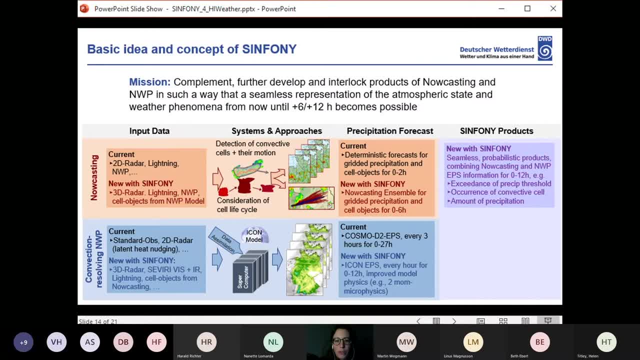 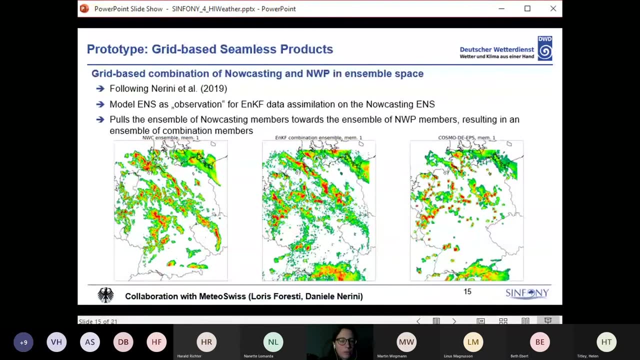 or also the most likely amount of precipitation that can be expected from a precipitating convective cell, And here is the first example on a grid based seamless product. So this is a combination followed by the method that has been developed by Daniel Nerini in 2019.. 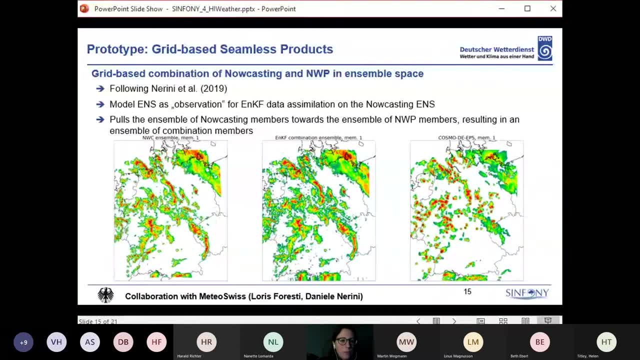 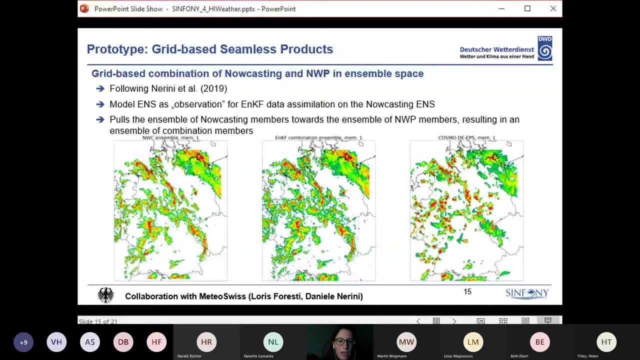 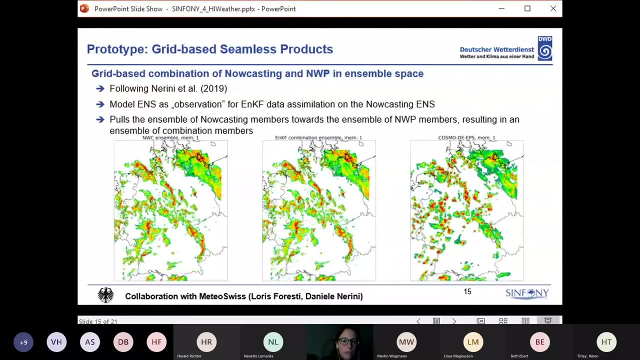 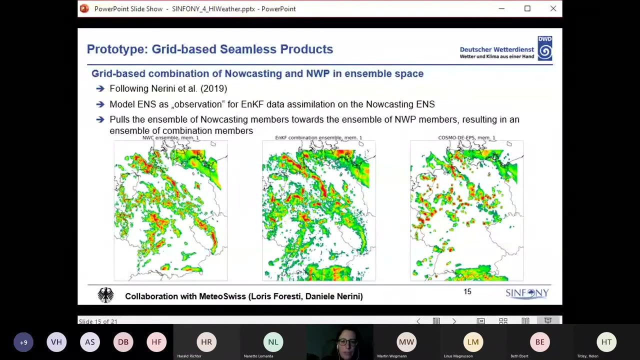 He is working at Meteo Suisse And for this combination the model ensemble is used as an observation for an ENKF data assimilation on the now casting ensemble. So it means that the ensemble of now cast is pulled toward the ensemble of NWP members with progress and time. 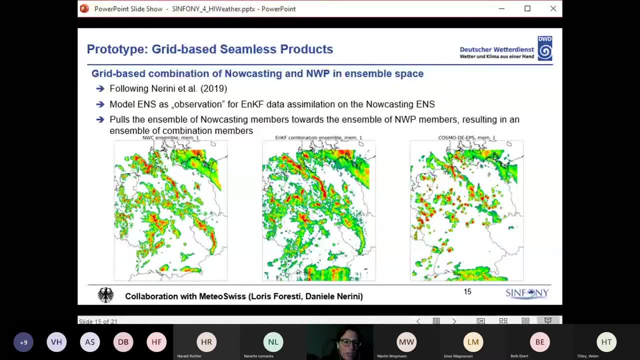 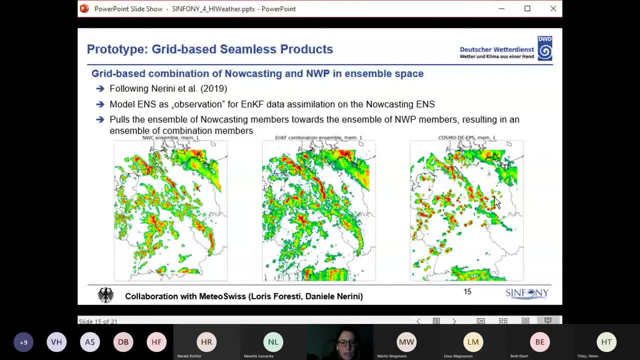 And this results in an ensemble of combination members. On the left hand side you see the now casting ensemble member. On the right hand side you see an ensemble member from the COSMO at that point still, And in the middle you see kind of this transition between the now casting. 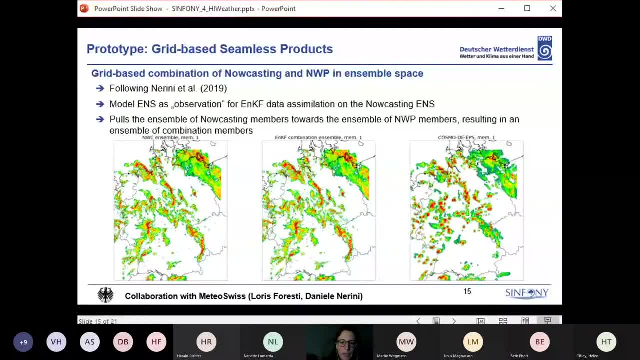 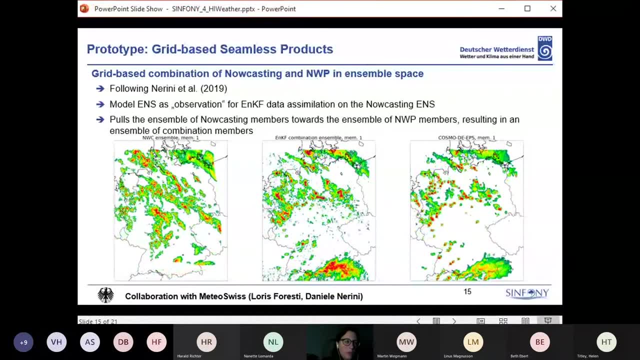 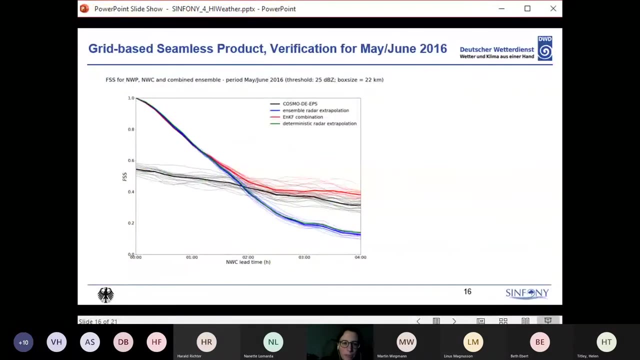 and COSMO model. So this is just the first example. We are also working on other techniques here And we also work on a seamless combination of the object ensemble, object based ensemble. But that today, due to due to time, And when you remember the first plot I showed with the skill or the score. 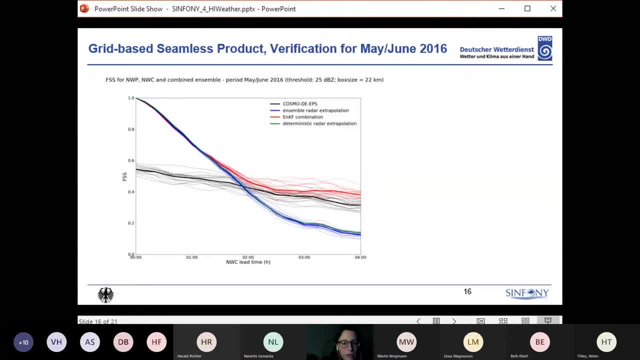 plot. we used to explain Symphony, So this is the first realization on how this could look like, or how this actually does look like at the moment. In black we see the COSMO EPS here. The blue is the radar extrapolation. So the now casting. 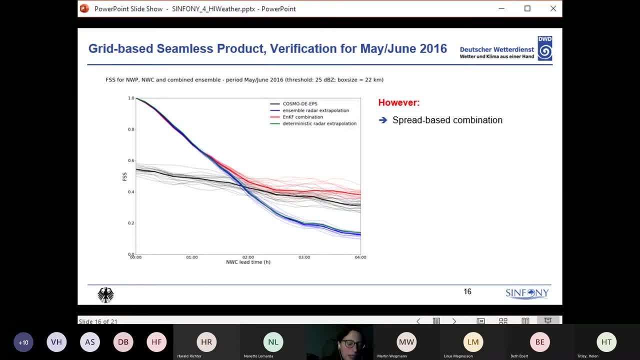 And the red is this ensemble filter Kalman ensemble Kalman filter combination I just explained, And so it's a spread based combination. It kind of puts together the best of both worlds, But the skill is not guaranteed And it works better for periods of decaying convective activity and less. 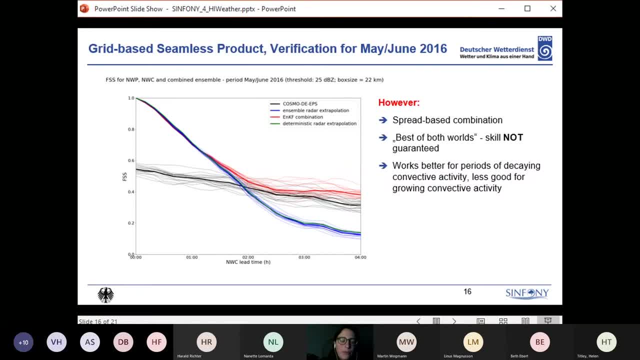 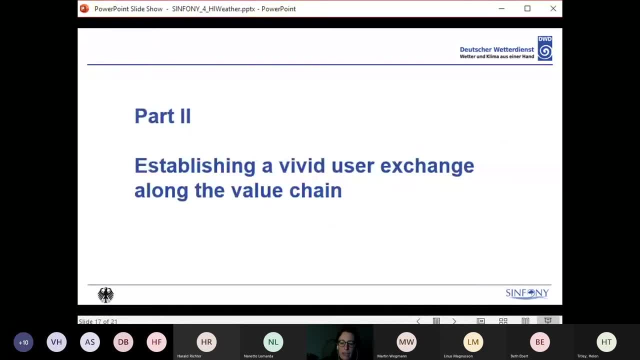 good for growing convective activity, simply because the growing aspect is not really Captured well yet. So that's part of of the symphony model And the second part of the presentation, which will be also shorter, briefly want to present on our work to establish a way with user exchange. 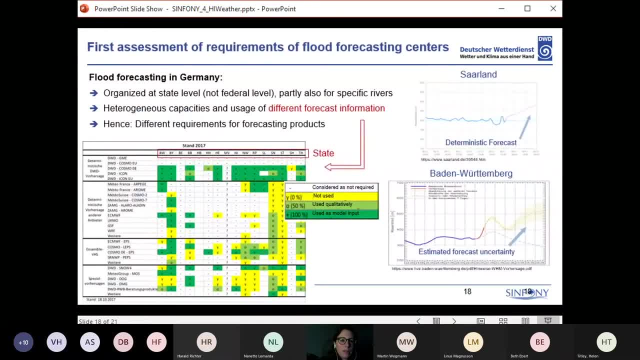 along the value chain. So one of our customers will be the flood forecasting centers in Germany, and the flood forecasting here is organized quite deeply Then in other countries. So it's organized on a state level, not federal. So in basically we have 16 different departments working on flood forecasting. 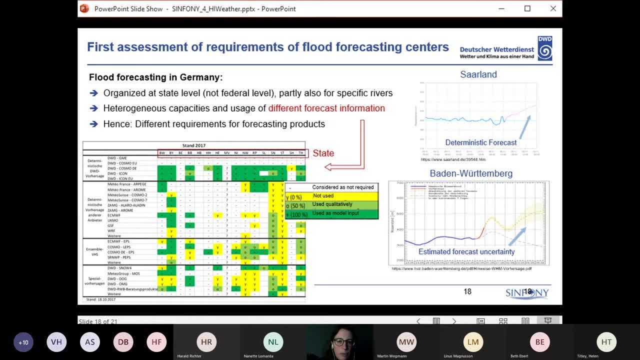 There are also other flood forecasting centers for specific rivers- I think for Ryan- And this also means that all of these flood forecasting centers have pretty heterogeneous capacity capacities and use different forecast information already. So down below you see a kind of overview on which kind of deterministic 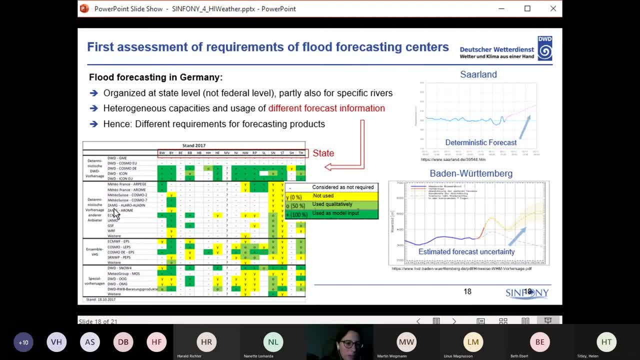 on the top from DWD. Other deterministic forecasts and ensemble forecasts are used by the different state flood forecasting centers. So you see some of them use ensemble forecasts, Some don't. In some cases there are only two people in this flood forecasting centers. 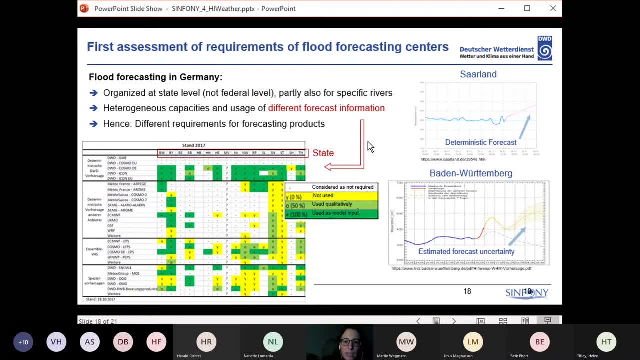 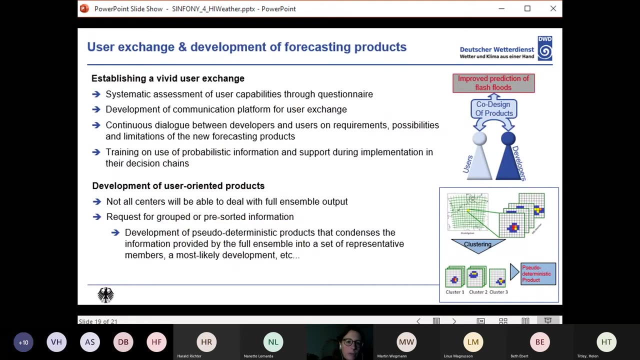 Others are pretty well equipped with stuff And also technical capabilities. Some do already provide forecast, uncertainty information and others don't. So this means we are focusing on a group that is pretty diverse And we are now working on establishing a user exchange with them. 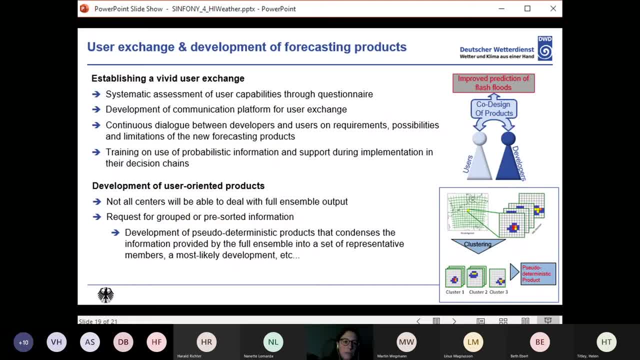 On the one hand, we are working on a systematic assessment of the user capabilities for a questionnaire. There is currently developed. also in collaboration with Vexicom from the Hans Ertel Center and Martin Goeber in Berlin, We are developing a communication platform for user exchange. 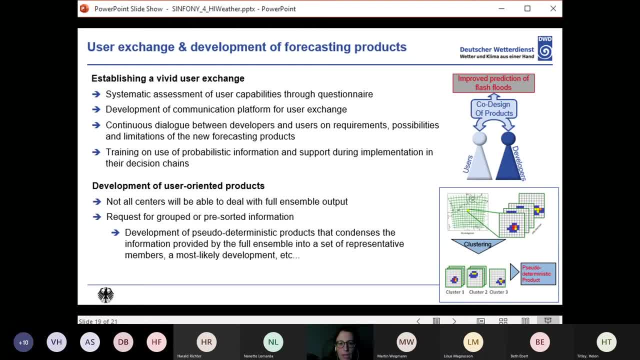 which can then also be used to provide examples of products and provide room for discussion. We are developing and establishing a continuous dialogue between developers and users on the requirements, the possibilities and limitations of the new forecast products. We also aim on running user workshops at one point when it's possible again. 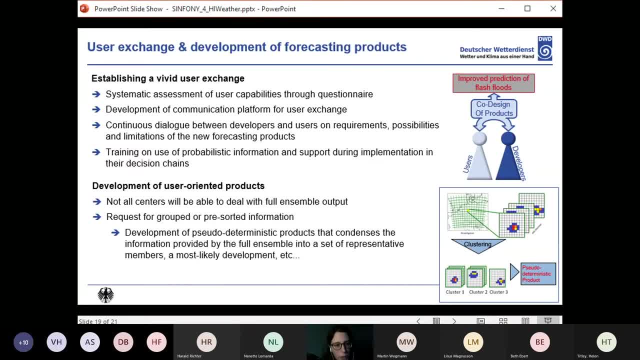 And another important component is also the training on the use of probabilistic information and support the users during the implementation of the new Symfony information into their decision chains. And due to the very diverse capacities of this flood forecasting center, it's also turned out that not all centers will be able to deal with the full. 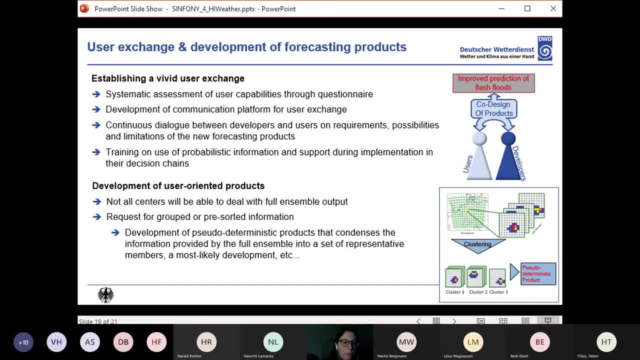 ensemble output, And they requested to get information that has been pre-sorted or grouped already. So this means that we develop so-called pseudo deterministic products that condense the information provided by the full ensemble into a set of, for example, representative members identifying the most probable development. 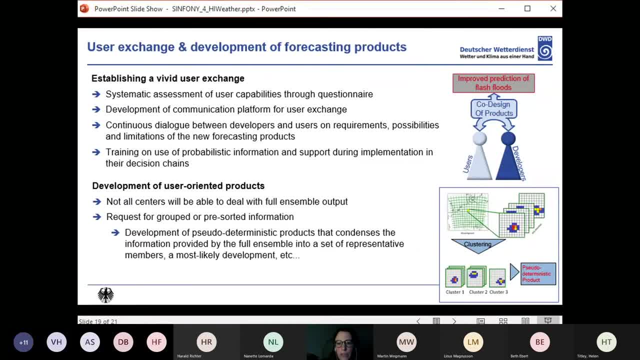 and so on. So the approach here is to explore different methods of clustering and then selection of representative members and so on. But this is work that has just kind of commenced and it's still in a pretty early stage, So I don't have anything concrete to show here at the moment.